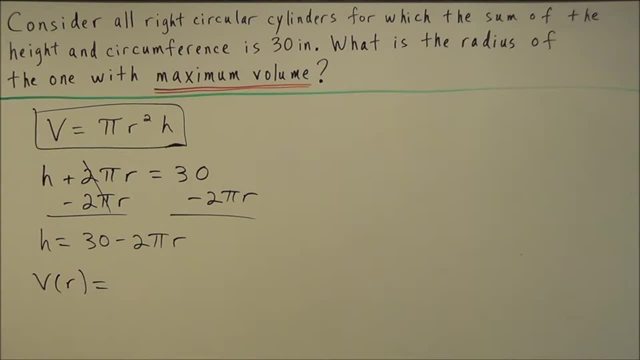 we're going to replace h with an expression involving r, So we'll have v of r equals pi r squared times h, which we could replace with 30 minus 2 pi r. So we could distribute here to simplify this And we'll have v of r equals 30 pi r squared. 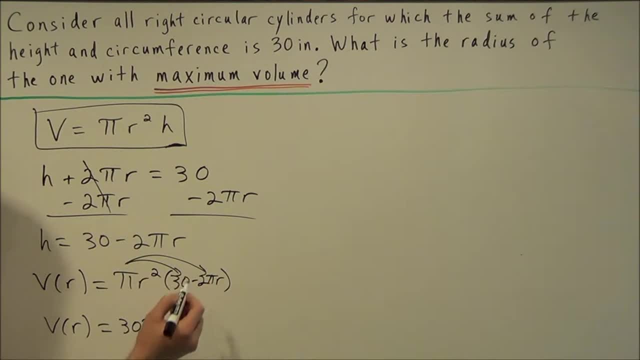 When we multiply the first two terms and we distribute to the last term, we're going to have minus 2 pi times pi is pi squared r. squared times r is r to the third power. So this is our function of one variable here that we're going to maximize. 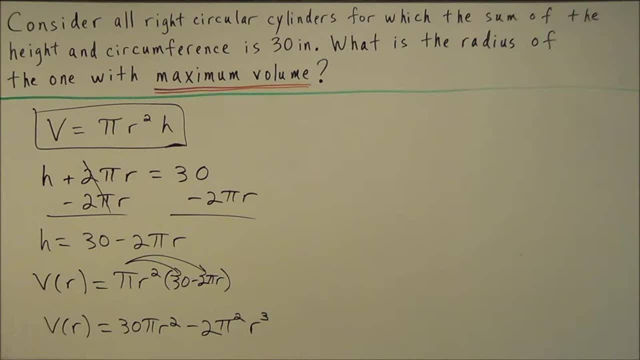 Now one of the things that we're going to do is: we're going to multiply this by the number of times pi squared. So, we're going to multiply this by the number of times pi squared. Now, one important thing is to consider the domain of this function, Considering that 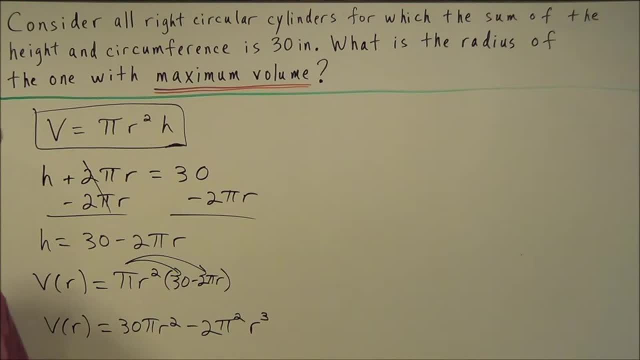 we're talking about a right circular cylinder. the radius has to be positive, So we need r to be greater than 0 for this problem. So this we're going to box off because this is a very important piece of information for solving this problem here. So next we're going. 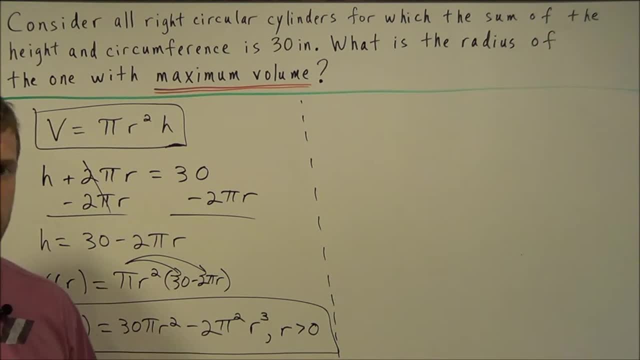 to use the concept to find an absolute maximum value. We need to use the concept of finding an extreme value. So we're going to take the derivative of our function. here We have v, prime of r equals and we're just going to use power rule. So we're going to have 2 times 30 pi is 60 pi. 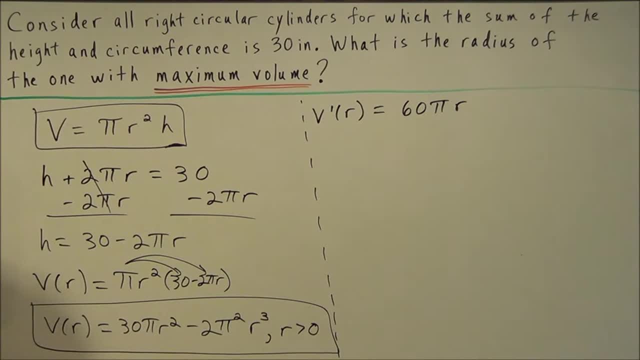 r to the 2 minus 1, so just r to the first power, And then we're going to use power rule on r to the third power 3 times negative. 2 pi squared is negative 6 pi squared, So we'll have negative 6.. 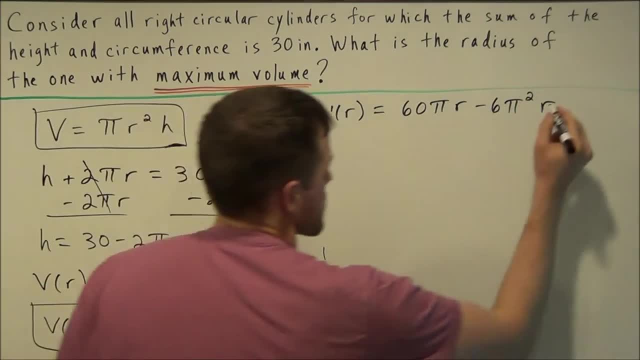 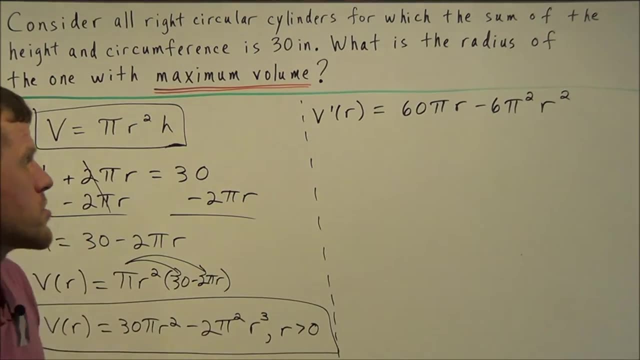 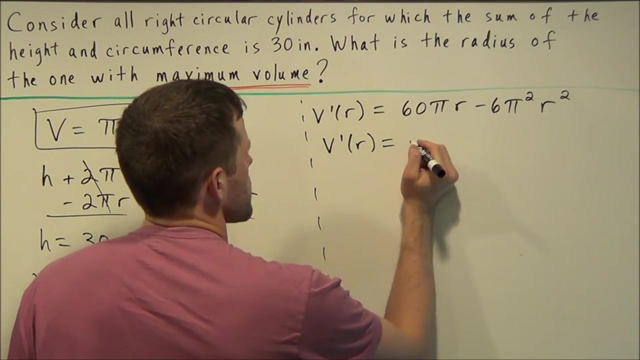 r to the third power 3 times negative. 2 pi squared r to the 3 minus 1 gives us r squared here. So next what we want to do is find the roots of this derivative here. So we're going to set v prime of r equal to 0. But what we should do first, before we set it equal to: 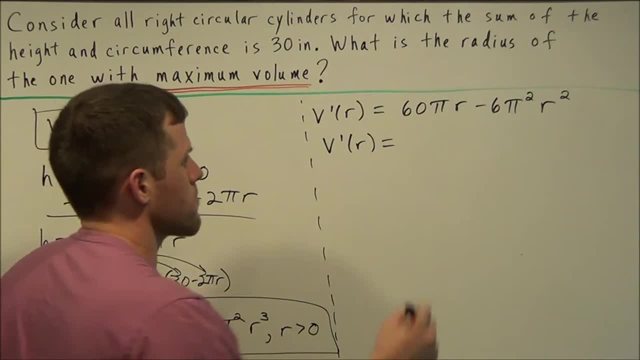 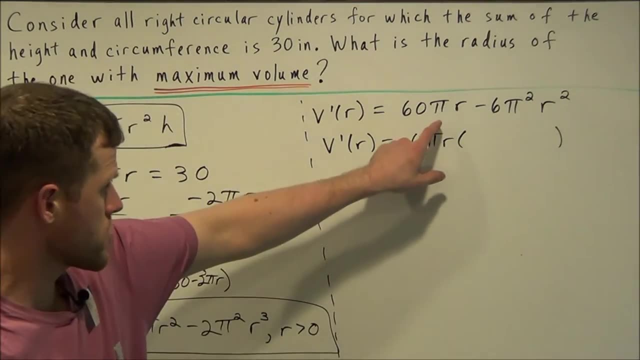 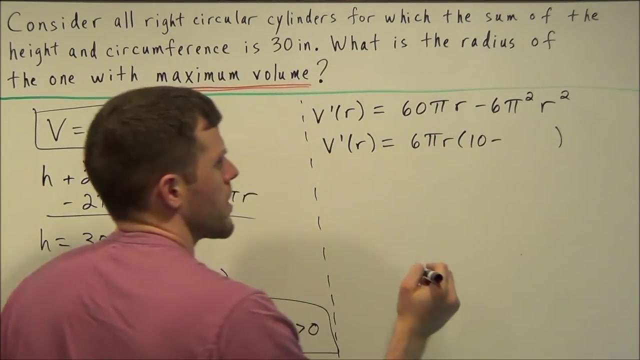 0 is, we'll factor out a greatest common factor. So for this problem here the greatest common factor will be 6 pi r, And if we factor this term out on the first part of this integral expression here we'll be left with 10, and then we'll have minus pi times r. Okay, so we're just 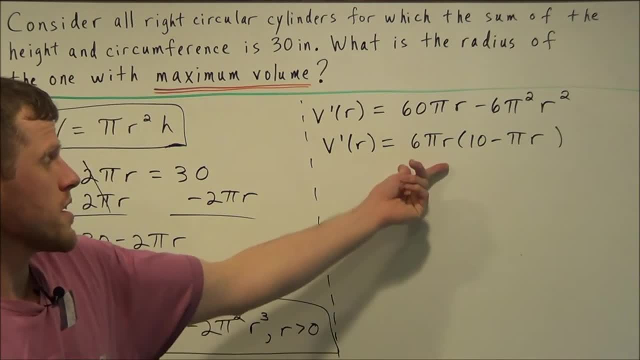 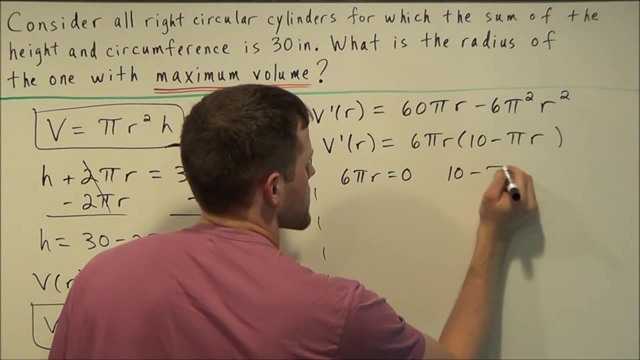 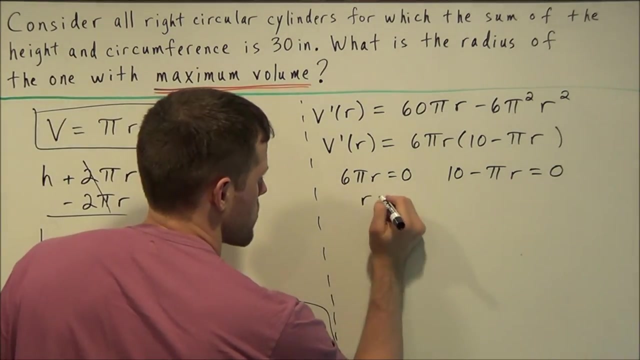 factoring out a GCF of 6 pi r. So setting this equal to zero, we're going to have 6 pi r equals zero and we'll have 10 minus pi times r equals zero. Now this first factor we could reject. This is going to give us r equals zero when we divide by 6 pi on both sides. but remember: 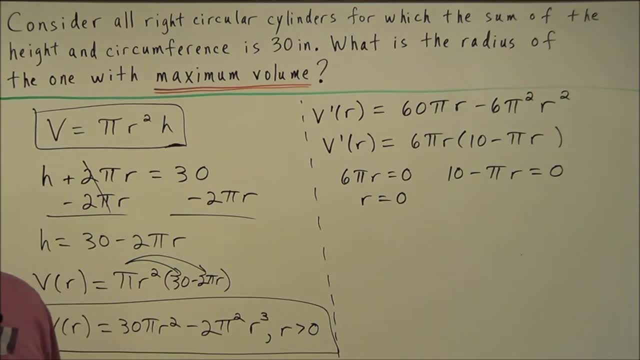 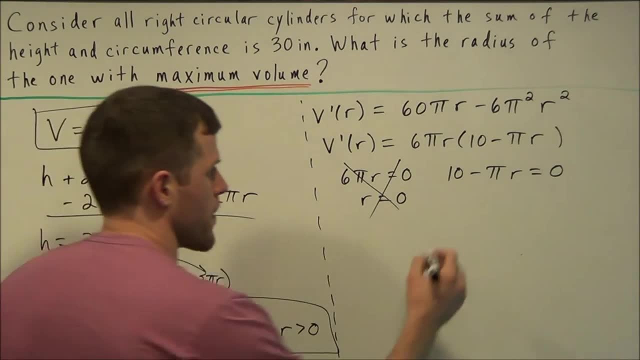 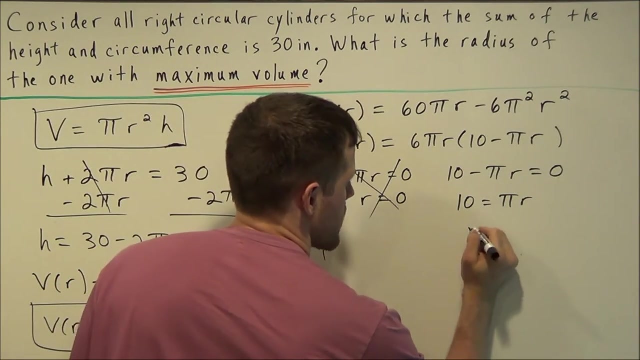 r has to be greater than zero. and think about it. We can't have a cylinder with radius zero. It would be non-existent. so we're going to reject this root here. However, the second factor is going to give us. when we add pi? r to both sides and divide by pi, it tells us r equals 10 over pi. 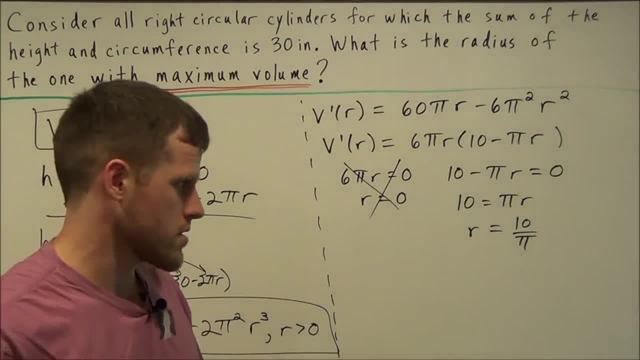 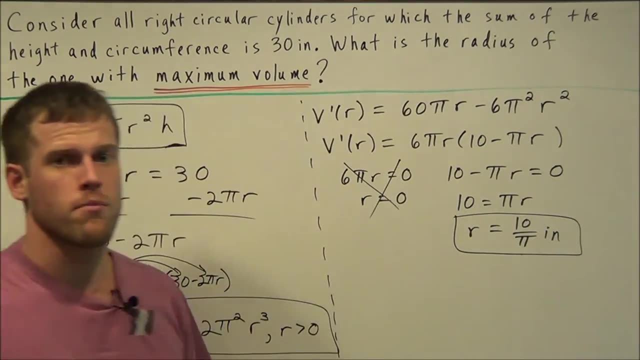 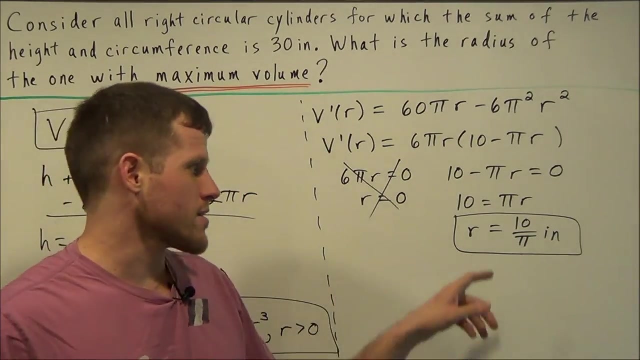 and if we want to throw the units in, we're talking about radius, which is a distance constant. This is 10 over pi inches. Now, before we close this problem out, this is the correct answer, but if you're not careful, you could fall into a trap that you have to check that this is actually. 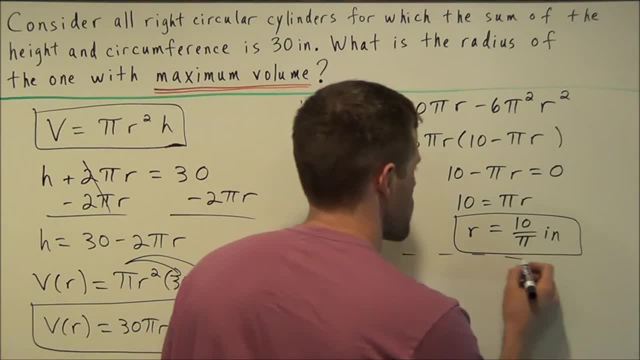 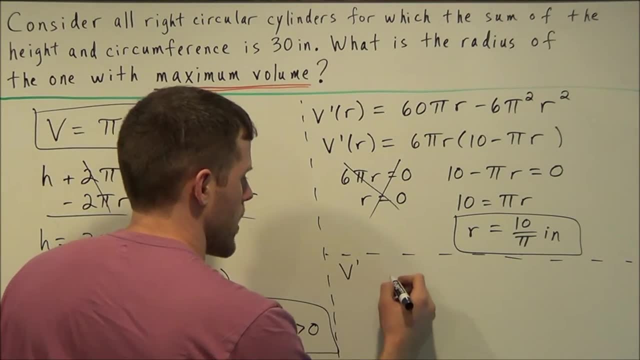 a maximum value of our function. So what you should do next is make a sine chart for the first derivative, v prime. So we have v prime and notice this sine chart is going to start at zero, and it could go on. So we're going to have a sine chart that's going to start at zero and it's going to go on to. 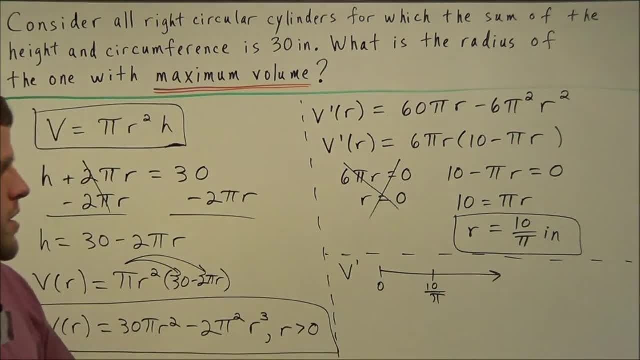 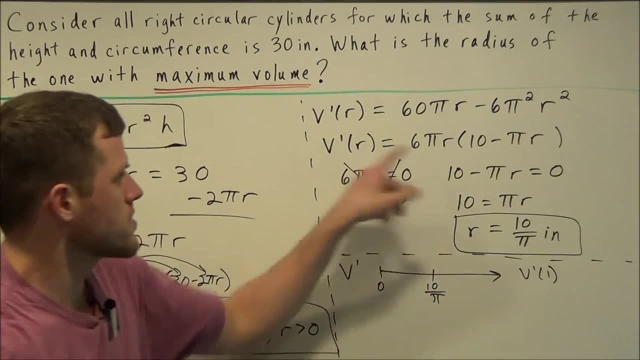 infinity and the critical value occurs at 10 over pi. Now if we plug in here, let's say we plug in something between zero and 10 over pi, If you plug in 1, you could plug it into the factored form. 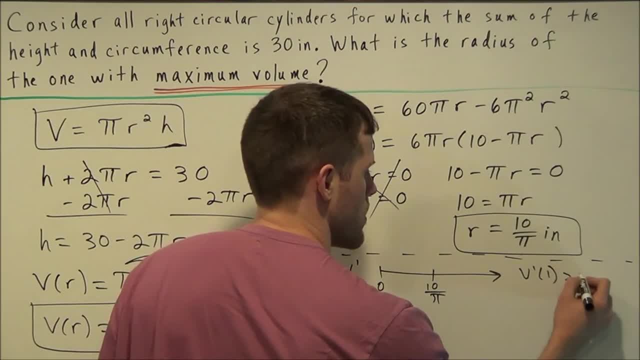 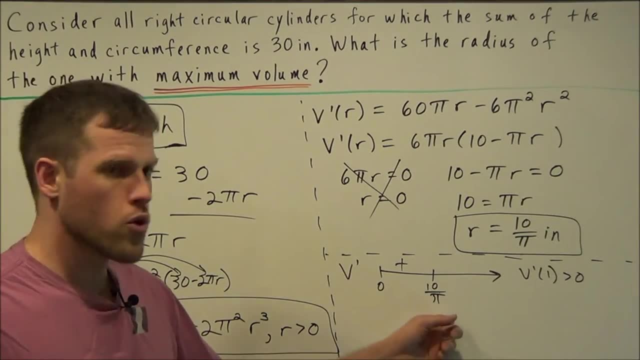 and it's going to give you a positive value here which allows us to label this first interval as positive. If you plug in something past 10 over pi, something like 4 or 5, you plug that into this factored form here and you're going to get a positive value. So you're going to get a positive value. 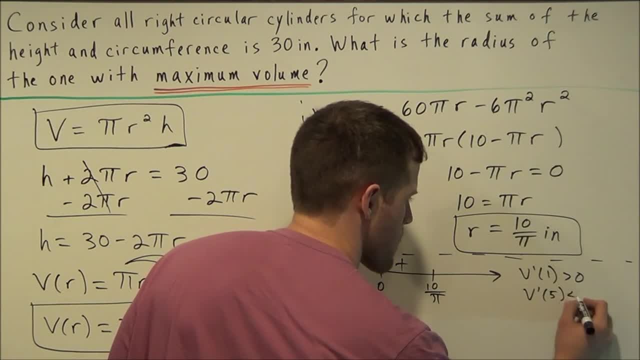 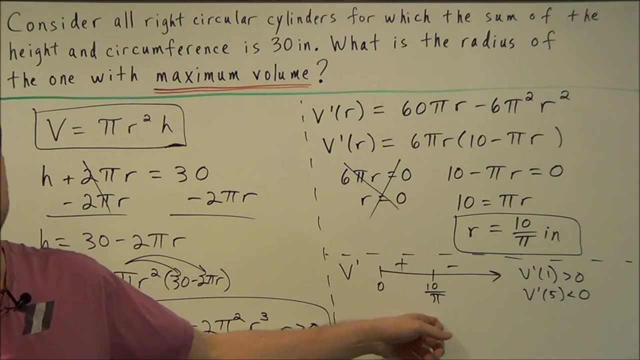 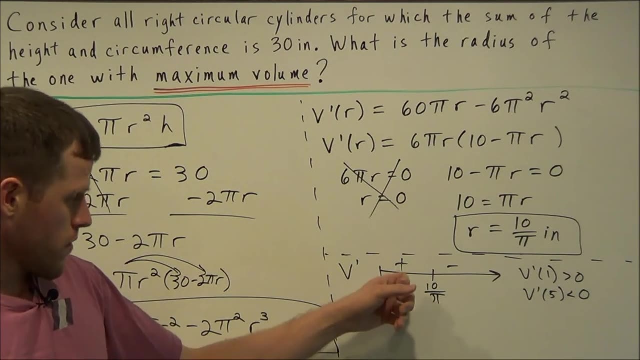 So you're going to get something negative here. So let's say, if we plug in 5, we're going to get a negative value And what this tells us? we can conclude that this is an absolute maximum because there's only one critical value and it's a local maximum. So if v is increasing from 0 to 10 over, 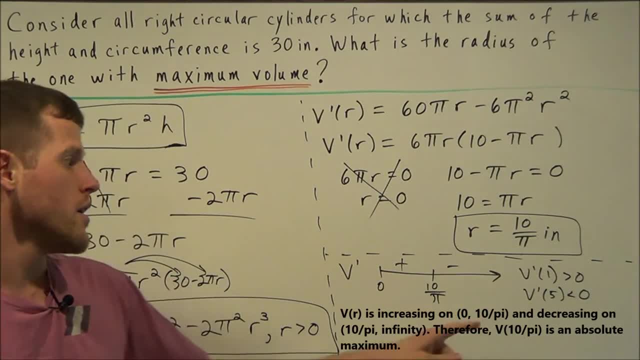 pi, and then it's always decreasing from 10 over pi to infinity. then that tells us that v of 10 over pi is an absolute maximum. So this radius is going to be negative. So if we plug in 5, we're going to get a negative value.